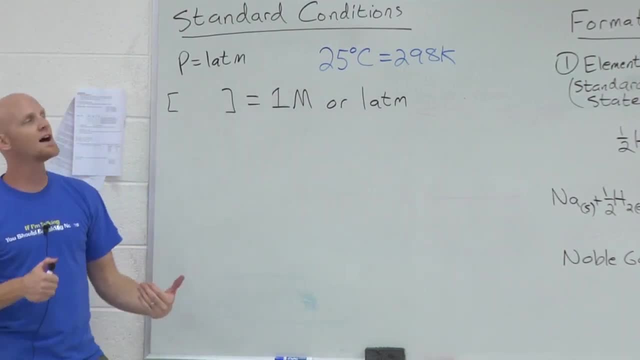 So this is different temperature than STP And again, it's really not technically part of standard conditions, but in gen chem it usually gets grouped in with it, So I'm going to throw it up there. Cool, these are your standard conditions. 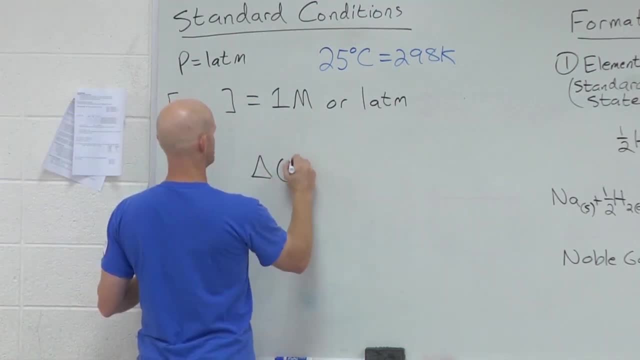 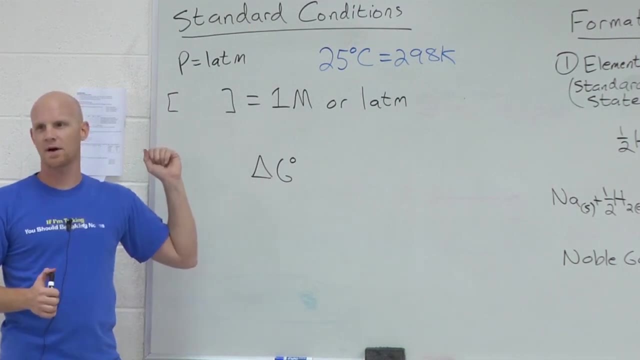 And so when you see delta G standard- that's the conditions that it corresponds to- You have one molar or atmosphere concentrations of all reactants and all products, equal amounts of both. So what if we're not doing a reaction under standard conditions? 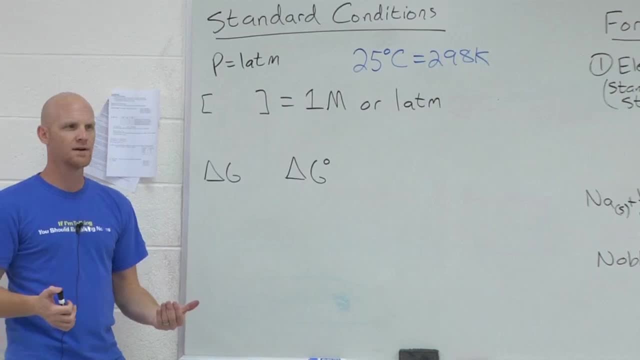 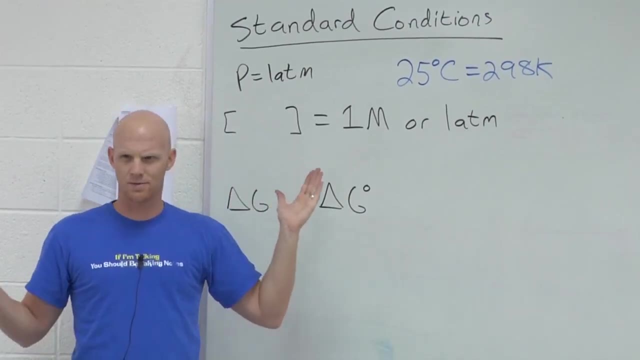 How often do you think you might do a chemistry reaction in a chem lab and start out with both reactants and products at exactly that concentration of one? Almost never, Almost never. But unfortunately this is the only set of conditions for which you typically find a bunch of published values. 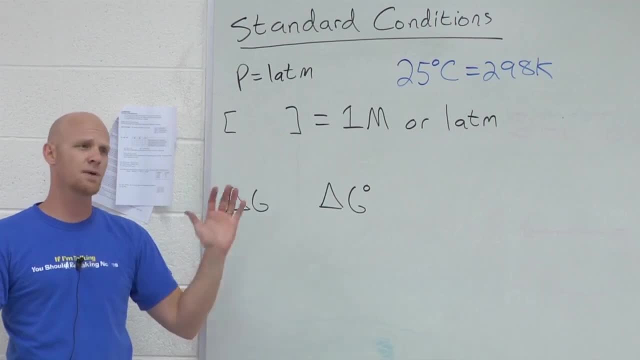 You can look up a whole bunch of reactions, Thousands and thousands and thousands upon thousands of reactions, And they'll give you values only for the standard condition. So what if you want to find out, well, what's delta G under some other, non-standard set of conditions? 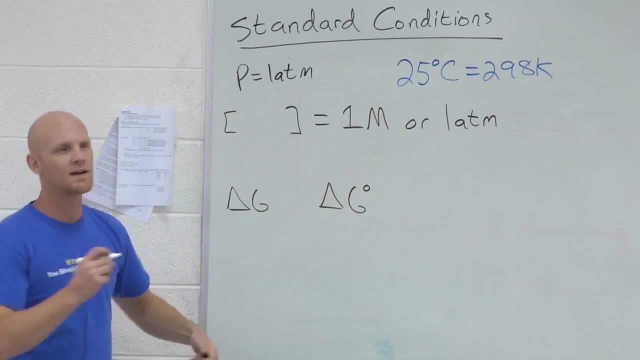 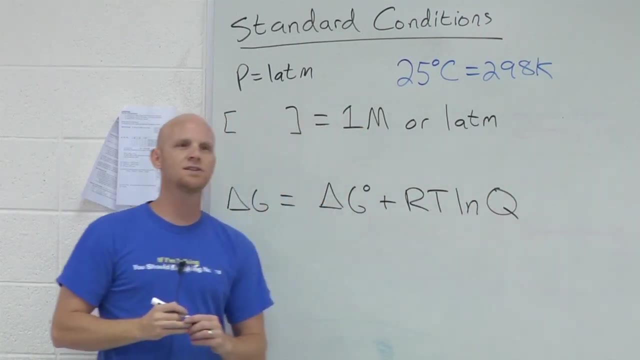 Well, you still look up that value in a book and then they tell you to add this fudge factor to account for any conditions that are not standard. You can put in a different temperature, and then Q, the reaction quotient products over reactants. 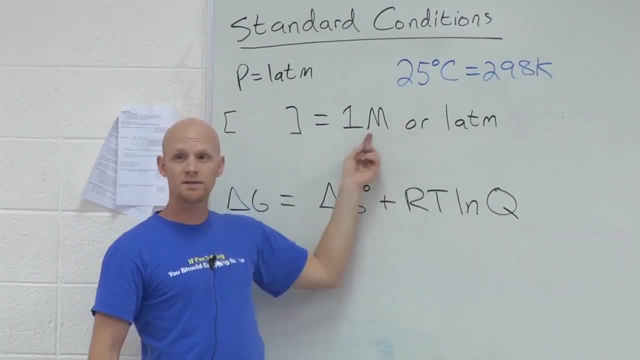 You can put in all the concentrations And so if they're not, one that'll get factored in Notice. what if you were under standard conditions and all reactants and products had concentrations of one? What would Q be under that case? 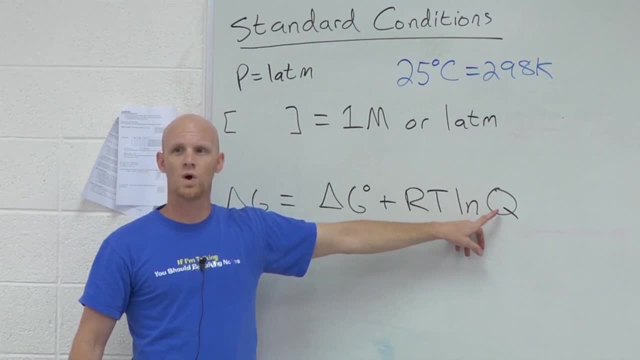 If all reactants and products were one, then Q would be also equal to well, it'd be one over one, which is one, And what's the natural log of one, Zero. And under those conditions this second term would go away. 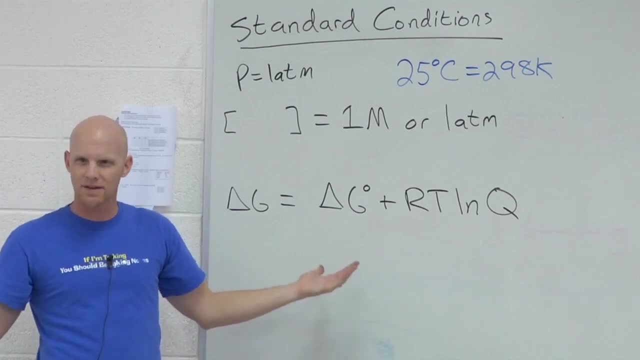 And your delta G would equal the standard value. So this kind of makes sense. Cool. So this is how you calculate delta G. when you're not under standard conditions, You've still got to use the standard value and look it up and whatever, but now you've got the rest of this as well. 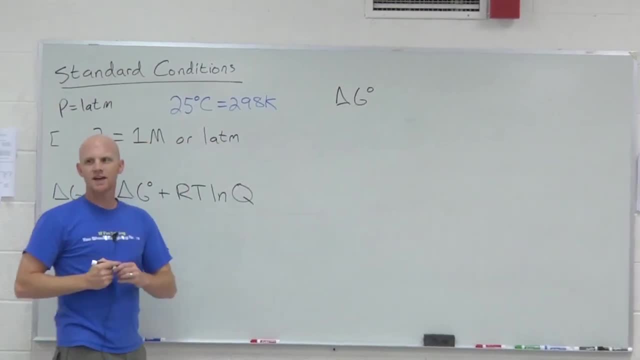 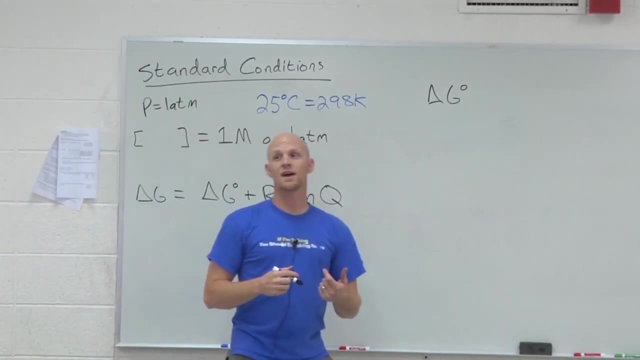 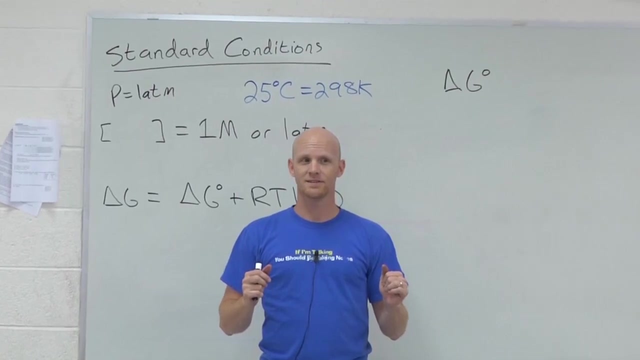 So we'll talk about delta G standard for another minute. here We can make some generalizations about delta G standard. So again, standard conditions. Do you have more reactants or more products at that point? Trick question, Trick question: Neither. 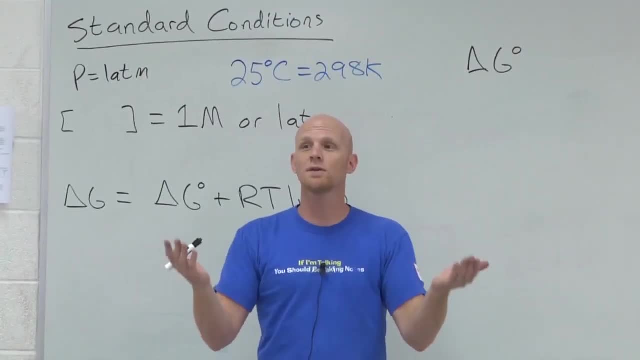 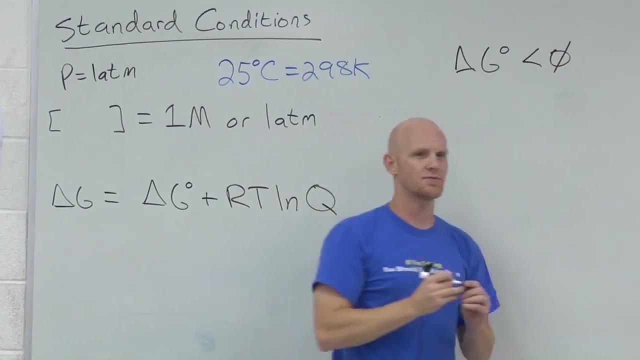 You've got equal amounts of both, right, Because everything's one molar or one atmosphere. So you have equal amounts, equal concentrations of reactants and products at standard conditions. So if I told you that delta G standard was negative, what does that mean? 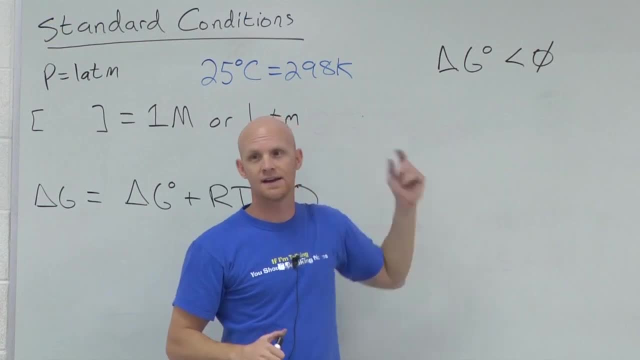 It means it's spontaneous at standard conditions. Is it spontaneous under non-standard conditions? I don't know. It might be, But this doesn't tell me about non-standard conditions. This little circle only tells me, then, about standard conditions. So under standard equal amounts of both, it's spontaneous. 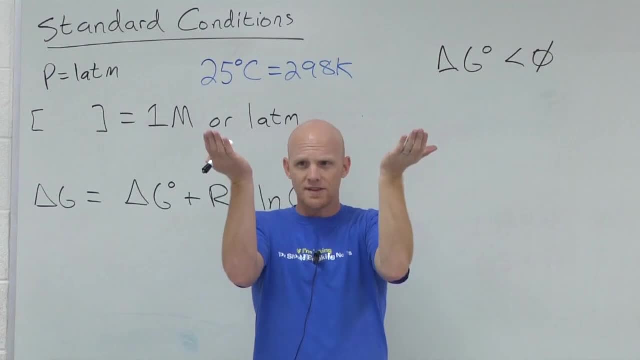 Delta G standard is negative. Okay, So if I start out with equal amounts of reactants and products at standard conditions and the reaction is spontaneous as it's written left to right, then I'm going to end up with more. what by the time I reach equilibrium? 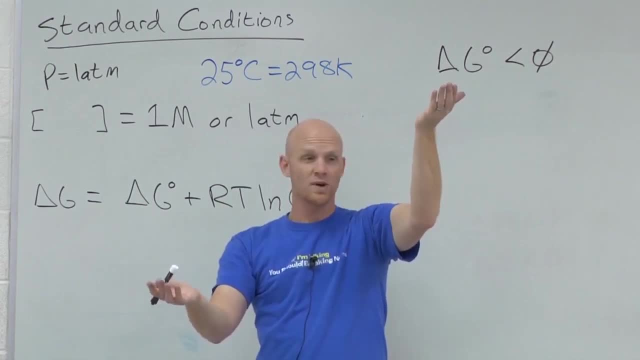 More products. under those conditions, And if, once I reach equilibrium, I have more products, then what should I expect for the value of the equilibrium? constant, Equilibrium, constant, Don't say zero, Because it's products over reactants and you've got more products than reactants. 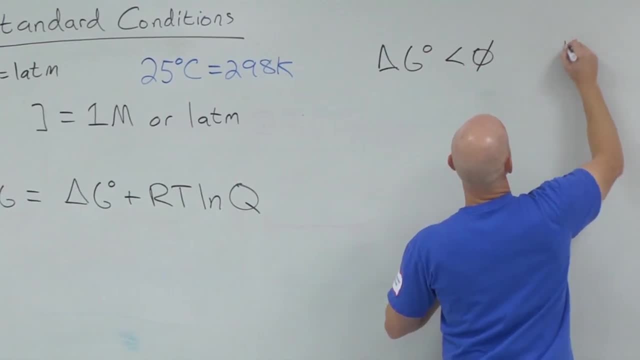 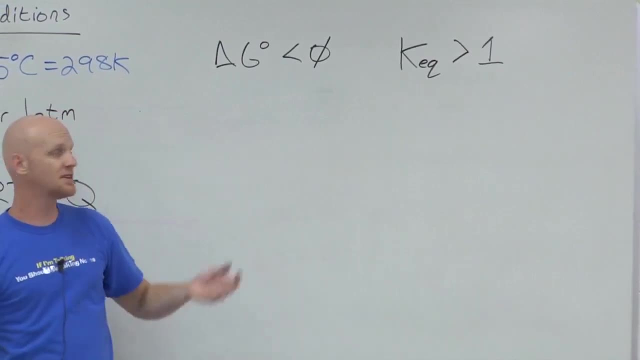 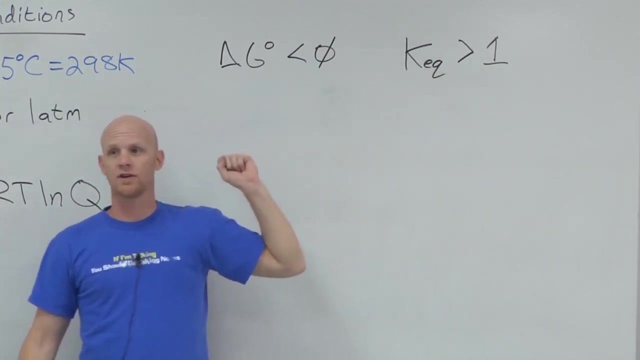 More numerator than denominator. All about one, not zero. So in this case, if delta G standard is negative K, your equilibrium constant will be greater than one. You'll have more products than reactants. That's a reaction that favors products. 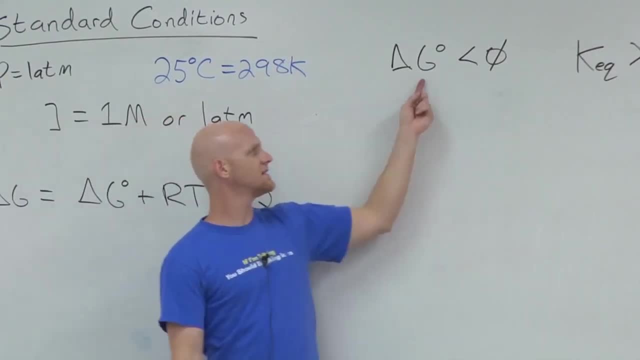 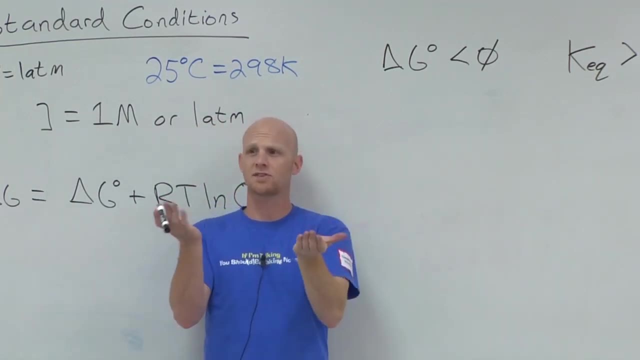 And this kind of makes sense in somewhat of an intuitive sense. I see delta G standard being negative and I should think, oh yeah, that reaction is spontaneous. Well, it's really spontaneous under standard conditions. But even if it's spontaneous under standard conditions, 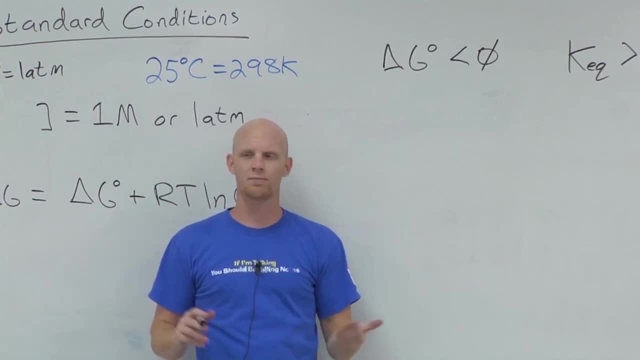 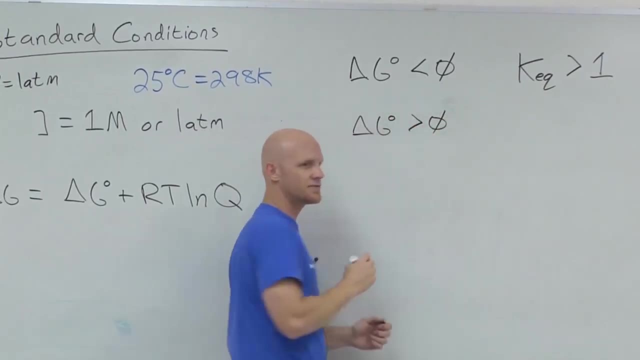 you should end up, when the reaction is done, at equilibrium, with more products, And so K is bigger than one, And you can say the exact converse as well. If delta G standard is positive, well, again standard conditions, you've got equal amounts. 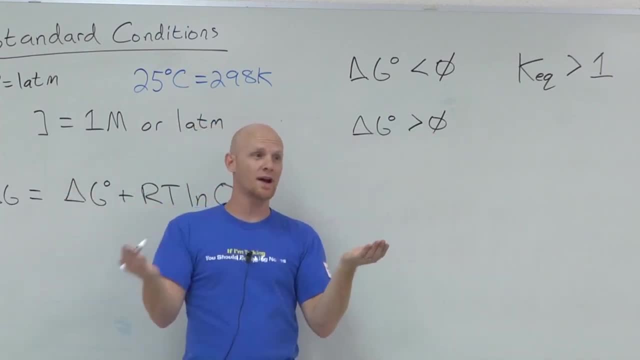 But if delta G standard is positive, then, as the reaction is written left to right, is it spontaneous? No, Under those standard conditions, it would actually be spontaneous going the other way, And so you'd end up with more reactants than products. 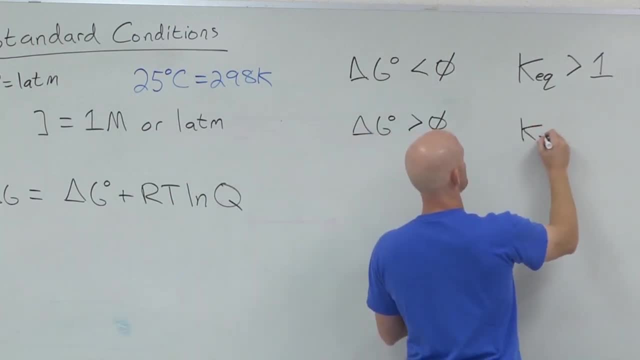 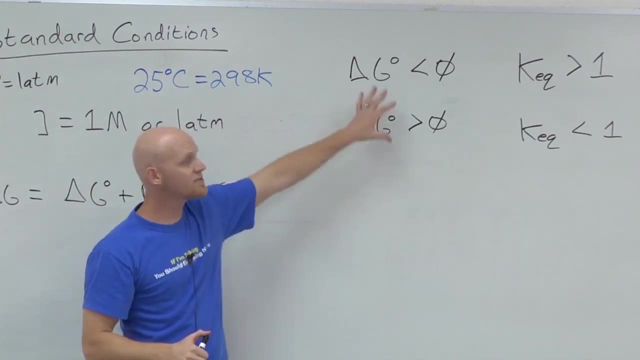 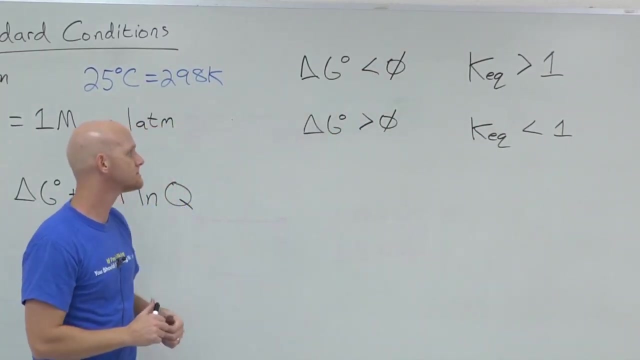 by the time you reach equilibrium, And in that case you'd therefore expect K to be smaller than one. So we connect this back to the equilibrium chapter. The whole equilibrium chapter is really a part of thermodynamics technically, Okay. So now that we've established that, 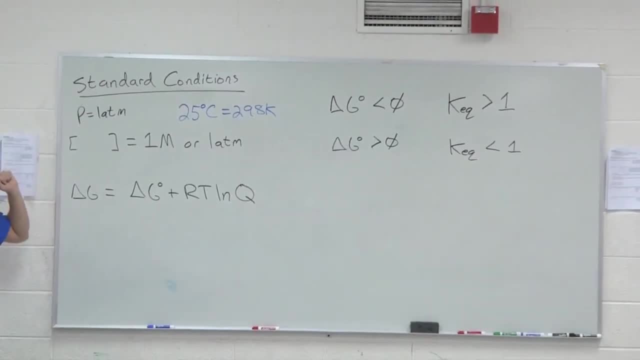 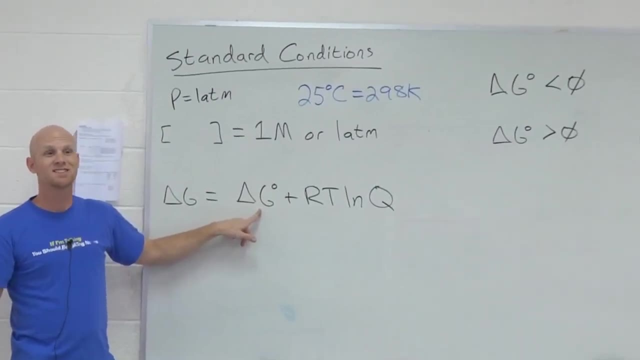 I want to come back to this equation real quick. So where do you get this value again? typically for a chemical reaction: In a book. You look it up in a book. So let's say I just happen to have a chemical reaction going on. 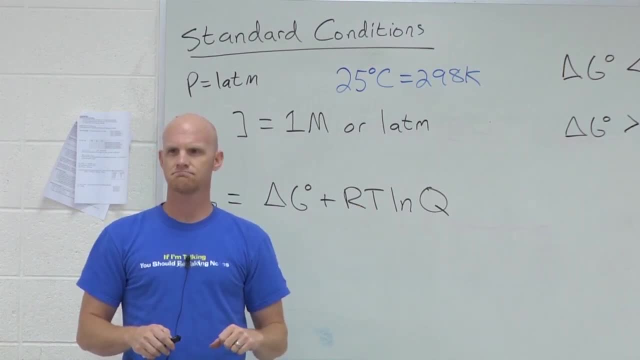 and I decided I wanted to start out at perfectly standard conditions. Okay, And so the delta G value for my reaction right when I started was exactly the number in the book. And then I let the reaction go And it turns out it was spontaneous. 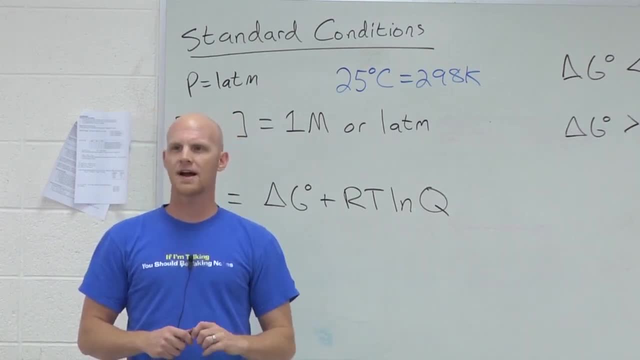 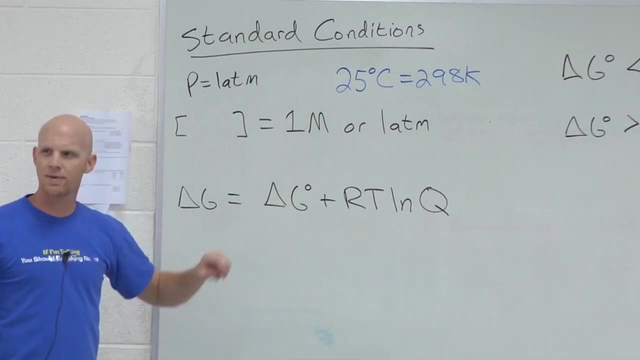 and so it goes, forming more products and using up reactants As that reaction proceeds. am I under standard conditions anymore? No, But if I look that value back up in the book, is it going to be a different number than I looked up the first time? 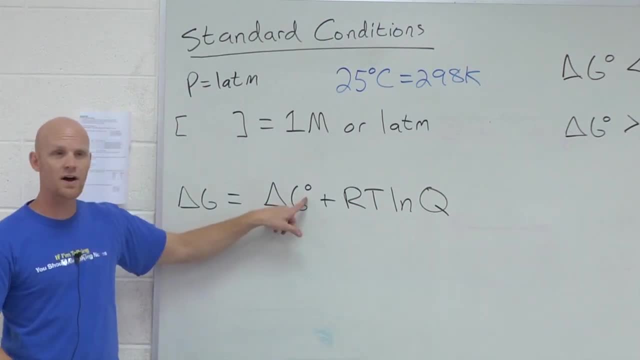 No, It's the same number. I'm not under standard conditions, so the value doesn't apply anymore, but it's the number of the book. This is a constant value for a given temperature. It's this value, though, that ever changes. 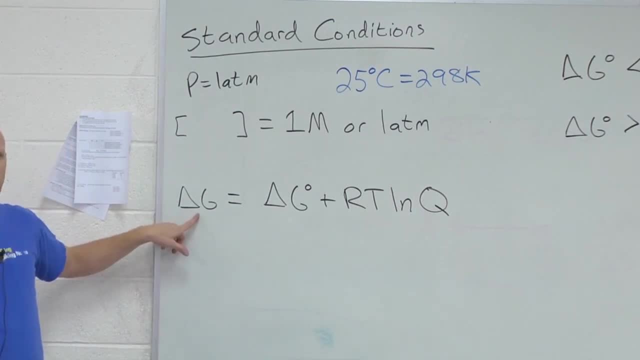 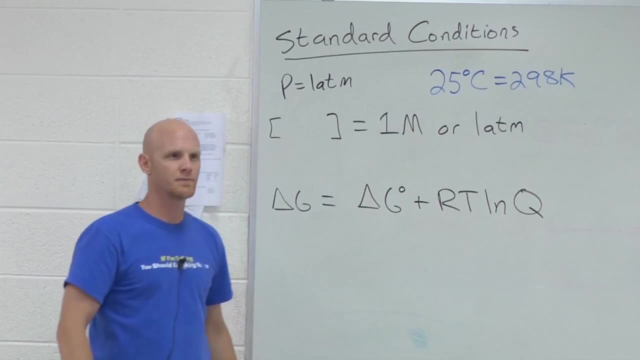 As the reaction goes on, this number is either going to get bigger or smaller, depending on if you know which direction the reaction's going and stuff like that. This is the one that changes. So when the reaction reaches equilibrium, will this number that you looked up in a book still be any different? 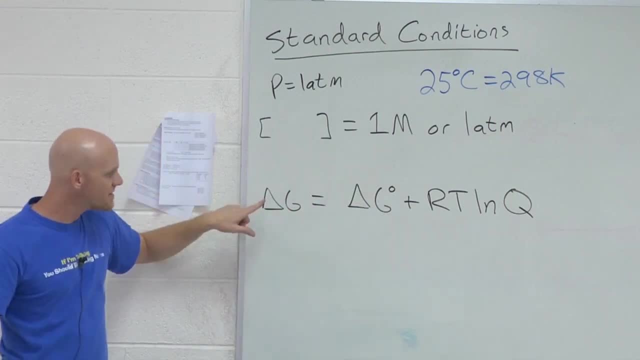 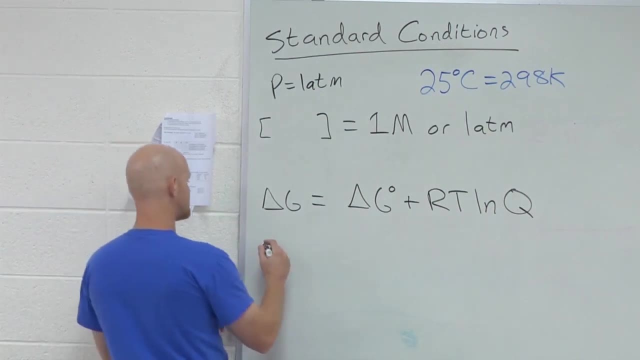 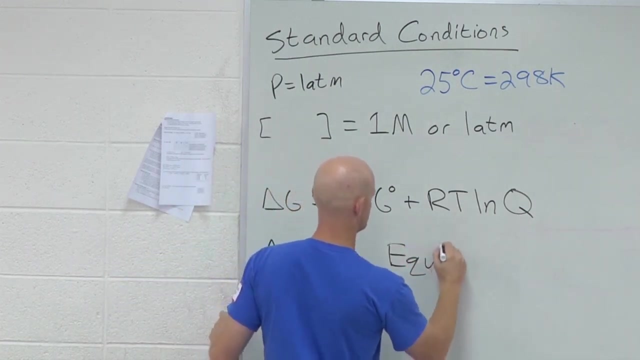 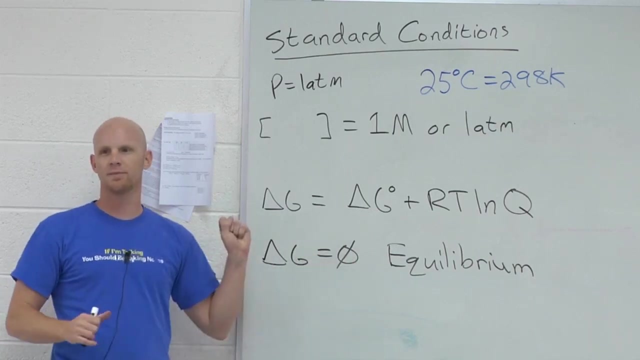 No, But when the reaction reaches equilibrium, this number is now what Zero. So in this case, it's when delta G, not standard value, it's when the non-standard value is going to hit zero. That's when you're at equilibrium. 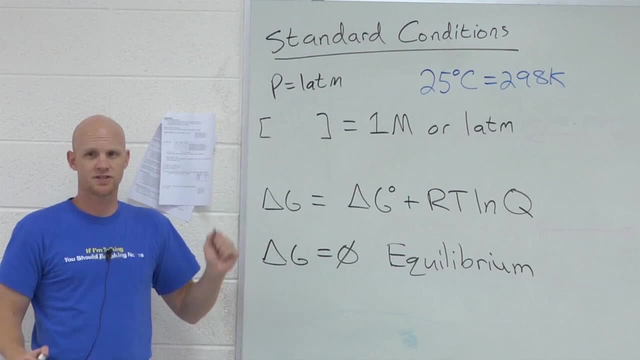 The standard value is what it is. You look it up in a book. It doesn't change for a given temperature. It's the non-standard value that's going to eventually reach zero once you've reached equilibrium. So if we look at this, then 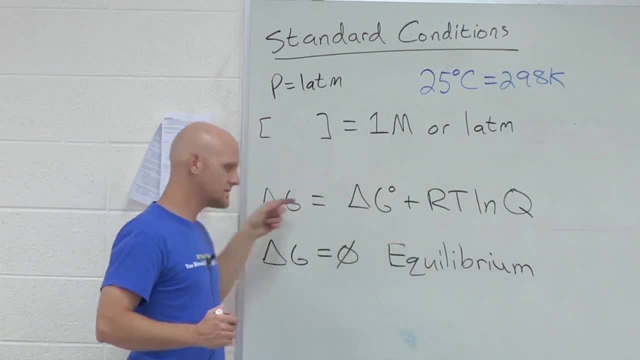 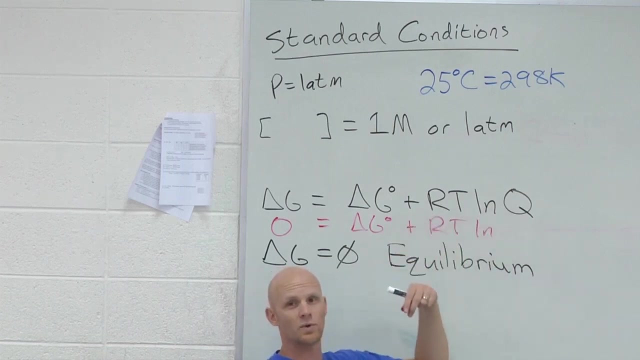 if it's this value that goes to zero, then this equation, a special case: when you reach equilibrium you'd get zero equals delta G standard plus RTln, And in this case, if you're at equilibrium, we can just say: Q is equal to what at equilibrium. 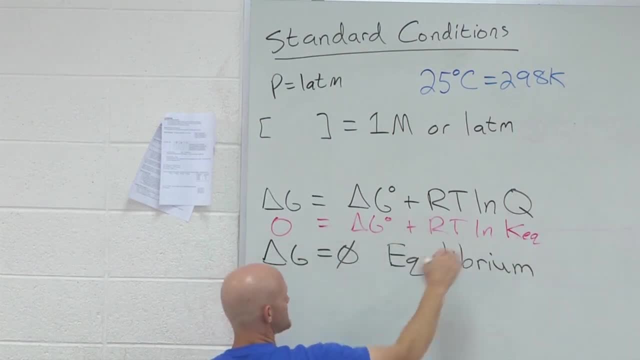 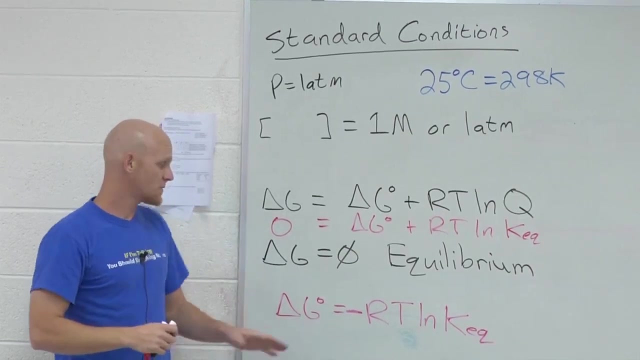 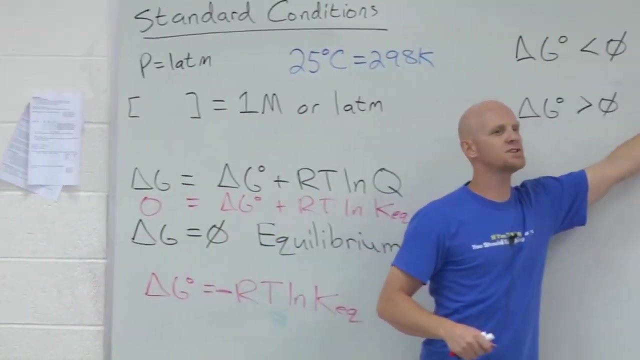 K, And if you rearrange this, you now find that delta G standard is equal to negative RT natural log of K. And so here is a mathematical formula for the relationship between delta G standard and Keq. It's the same relationship we just established. 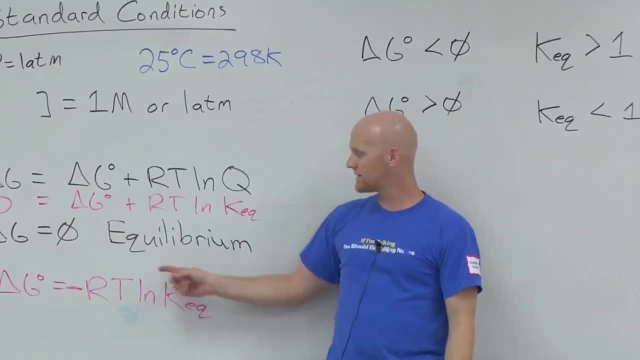 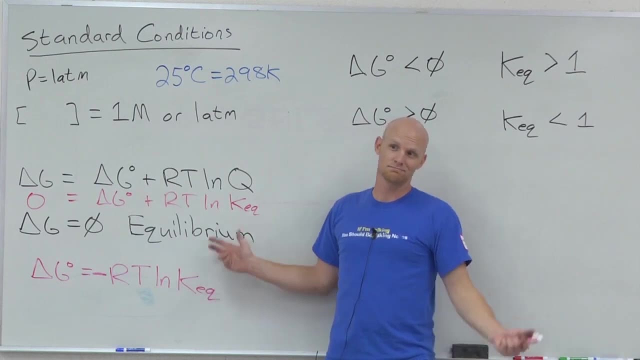 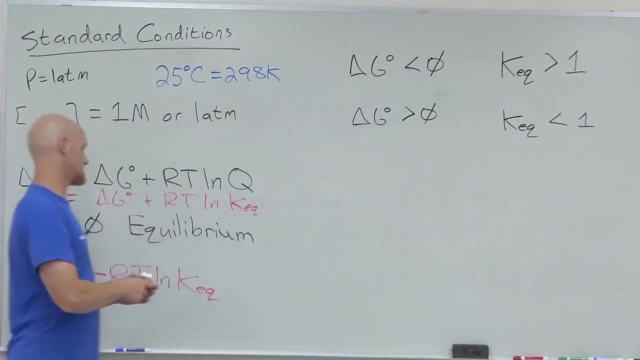 Here you can actually mathematically calculate things. If I give you Keq and a temperature, you can calculate delta G standard. If I give you delta G standard and a temperature, you can calculate Keq. Questions on that. One thing to note. 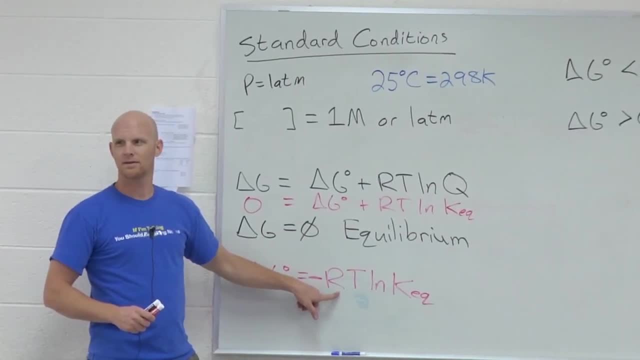 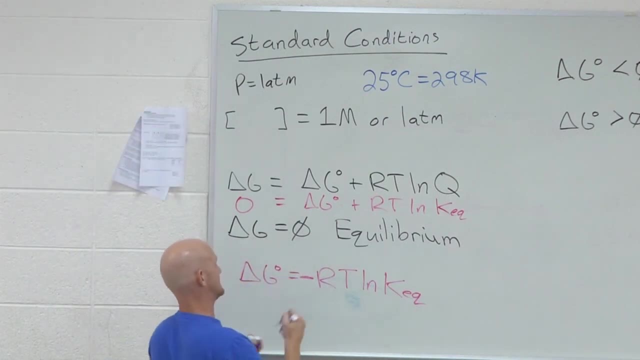 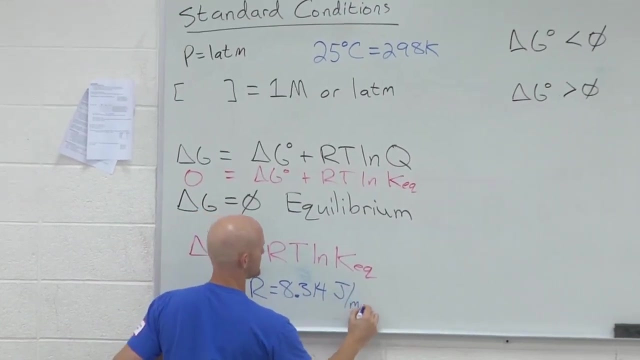 R here. What's that called? Anybody remember? Not a rate constant, but gas constant, Universal gas constant. In this case, the most common value you're going to have provided for you that's relevant to this chapter is 8.314 joules per mole Kelvin. 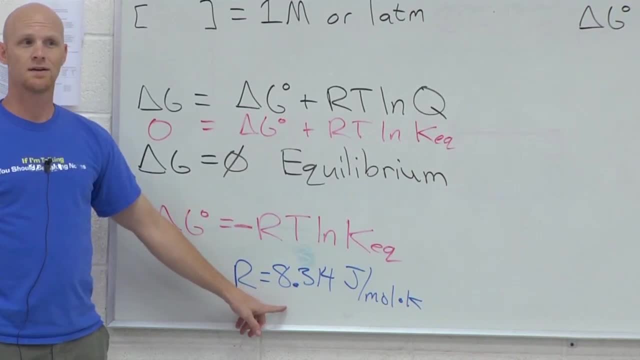 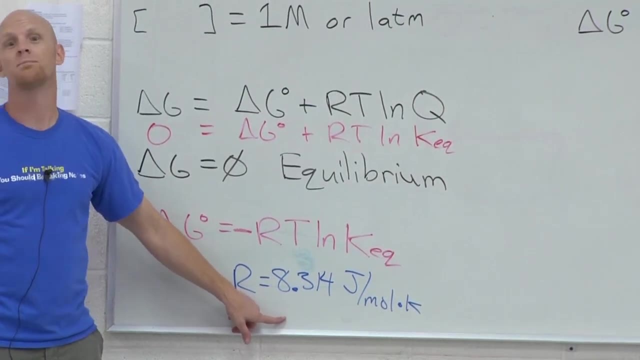 Unfortunately, this is not the only value they're going to give you, right? Where else did you see R originally? Yeah, PV equals NRT. Same R, But for PV equals NRT instead of joules per mole Kelvin. we're usually going to give it to you. 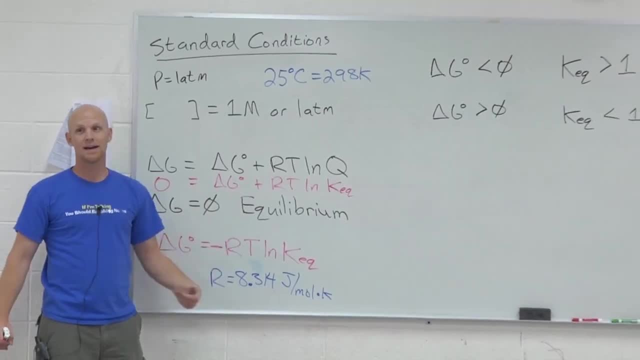 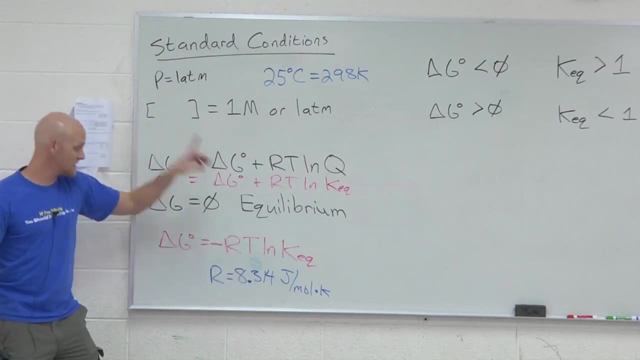 in liter atmospheres per mole Kelvin And expressed in those units it's a totally different number: It's 0.08206.. So you got to be careful. We're dealing with energy right now. Then you better use the R value.